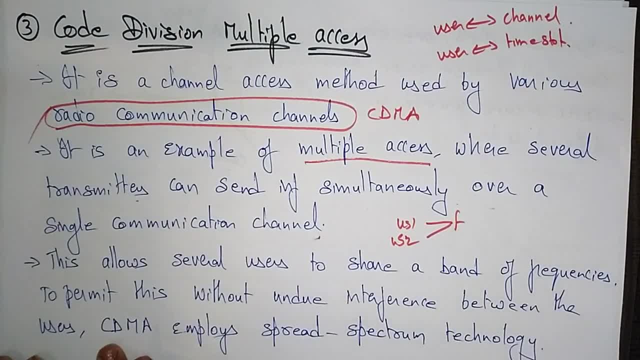 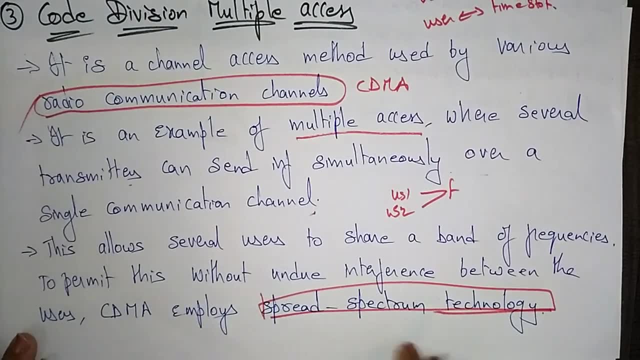 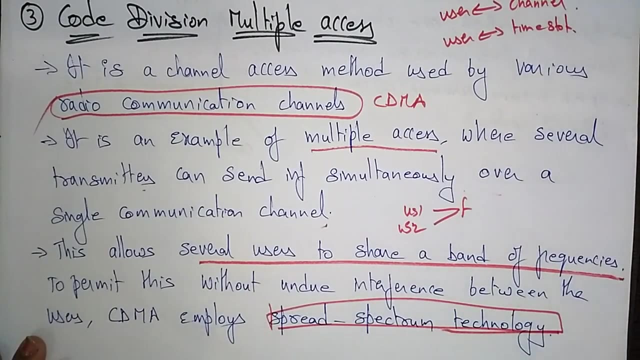 this without undue interference between the users. cdm may employ spread spectrum technology, so it's using the spread spectrum technology. why we call it as a spread spectrum technology? because it allows the users to share the band of frequencies. so it is sharing the band of frequencies. so it is. 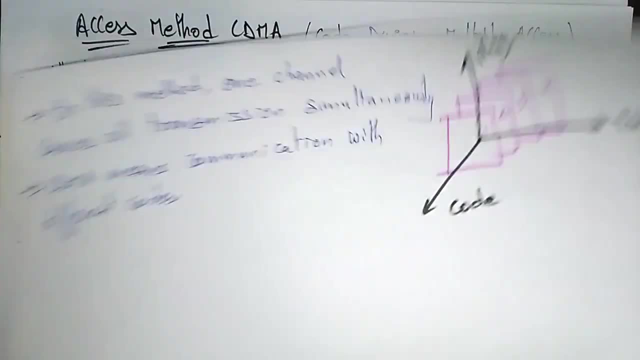 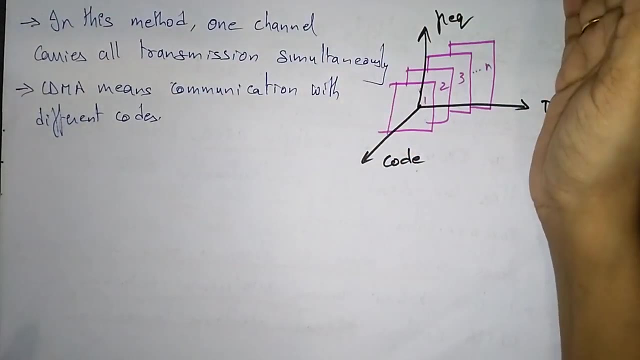 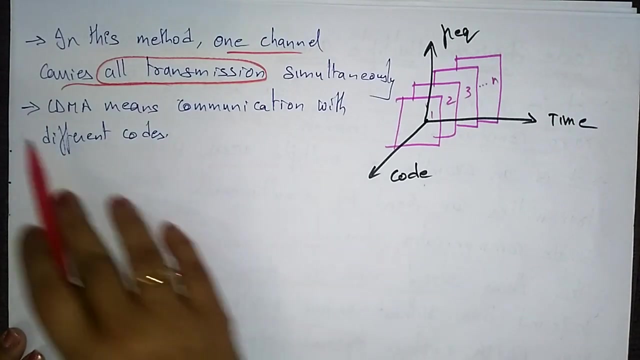 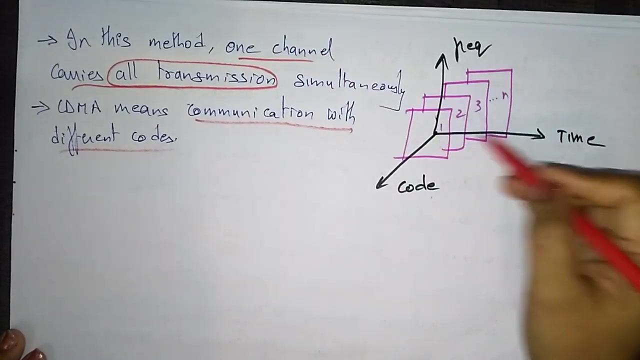 a spread spectrum technology. so in this method one channel carries all transmission simultaneously, not one channel will to one user. so here one channel carries all transmissions simultaneously. and cdma means a communication with different codes, a communications with different codes. so here rather than two, here three will be. this time code and the frequencies of cdma is a combination. 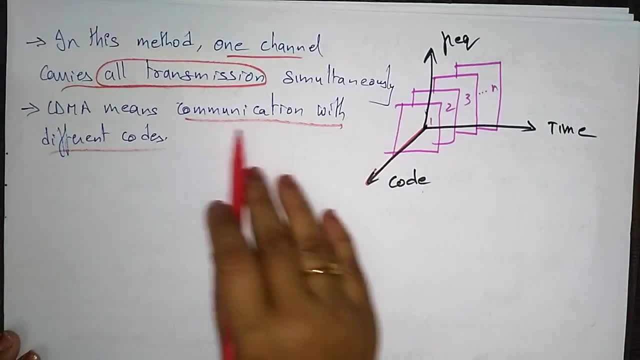 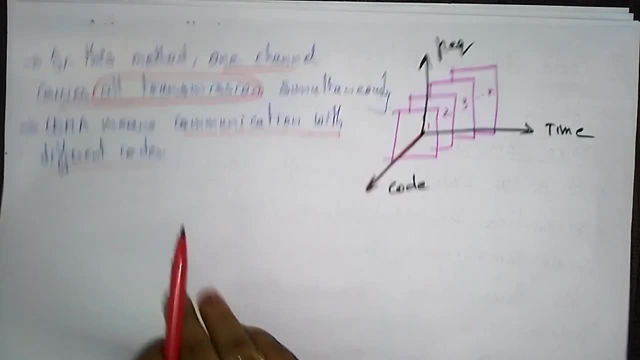 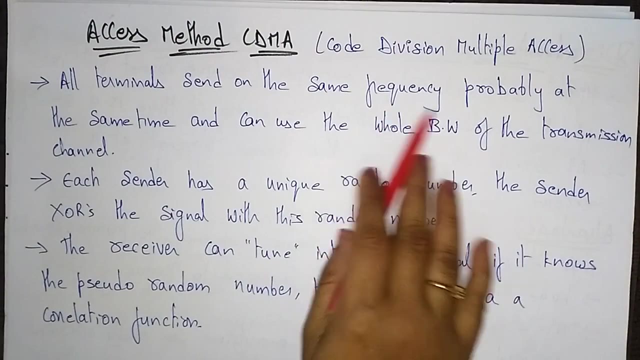 of both fdma and tdma. uh, it pro it means the communication with the different codes. okay, so let's see what is this. access methods of the cdma. the access method of the cdma: here all terminals sends to the same frequencies, probably at the same time, and can use the whole bandwidth. 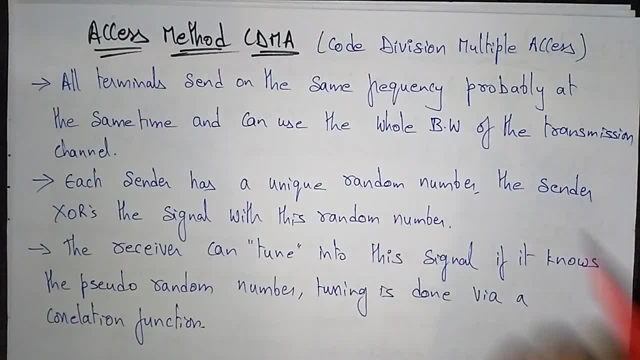 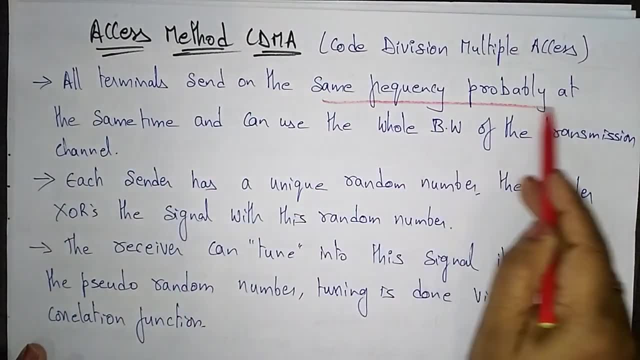 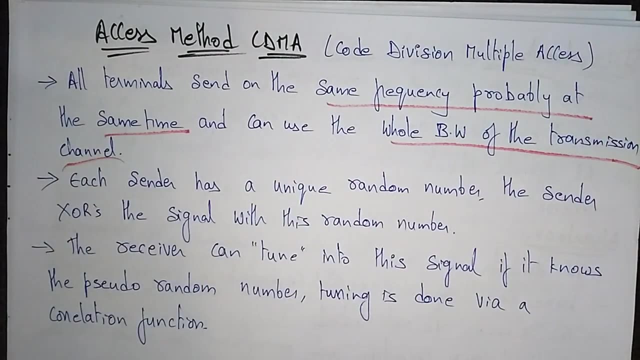 of transmission channel. so i said it's a combination of frequency plus time. so here, all terminals, whatever. it is there that the devices sense on the same frequencies, probably at the same time. they can send at the same time and can use the whole bandwidth of transmission channel. each center has a unique random number. the sender exhausts the signals. 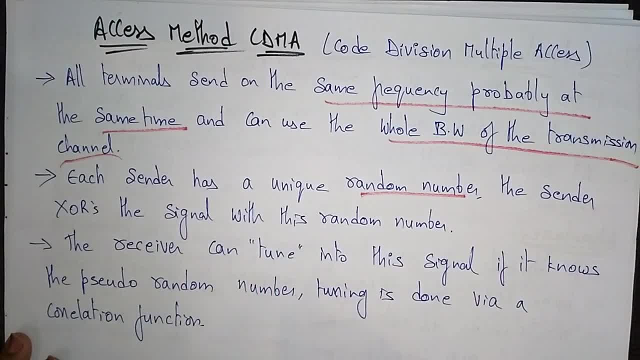 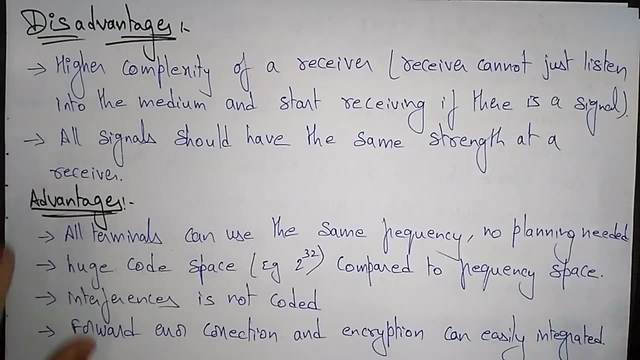 with it with this random number and the receiver can tune. so whatever the receiver that is receiving, that receiver can tune into these signals if it knowns to pseudo random number tuning is done via correlation function. so now let us see the disadvantages and advantages of cdma. 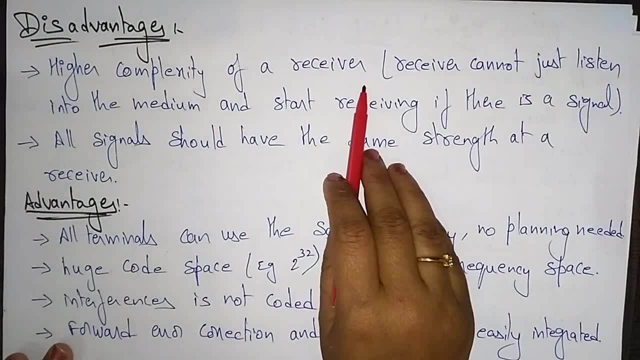 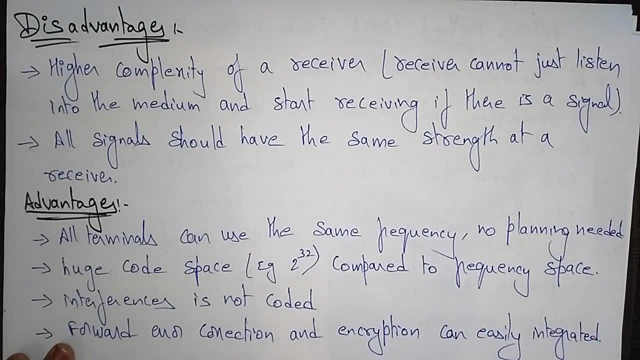 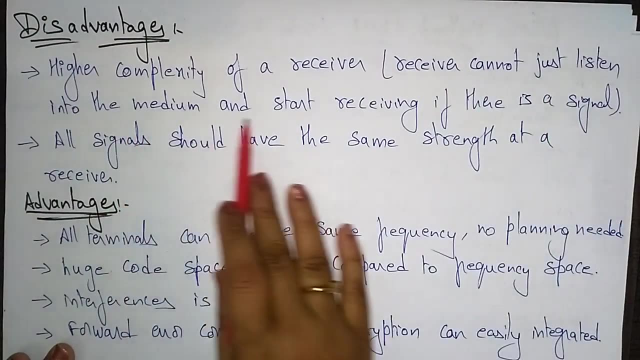 the disadvantages are higher of a receiver. that is, the receiver cannot just listen into the medium and start receiving. if there is a signal, okay, it's not simply receiving listening the signal, it's whenever it receives the signals- uh, here, the uh, the medium- and start receiving. if there is a signal, all signals should. 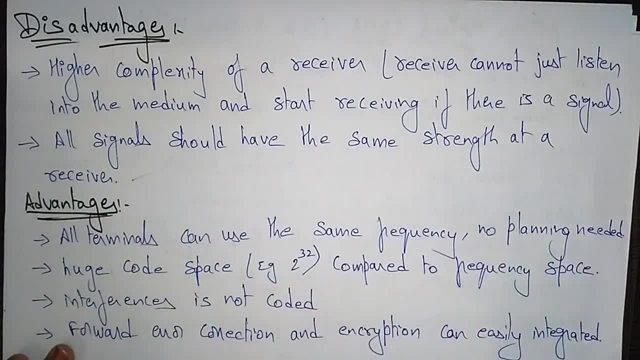 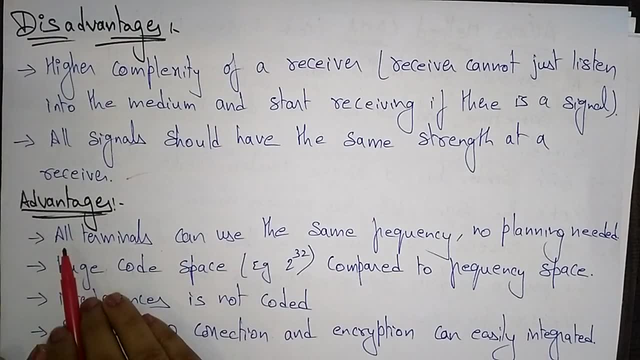 have the same strength at the receiver side, so that you call it as a disadvantages, because all signals are having the same strength at the receiver side and the advantages is all terminals can use the same frequency. no planning is needed and huge code space will be provided by the cdma. 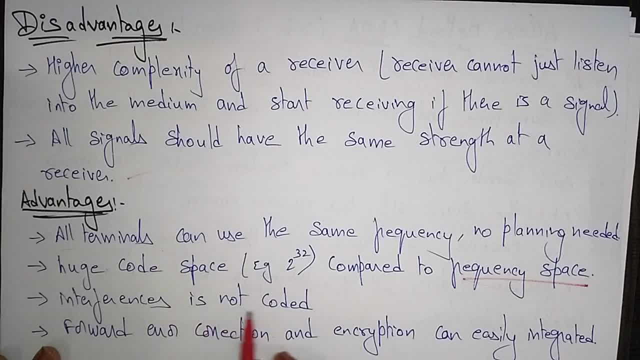 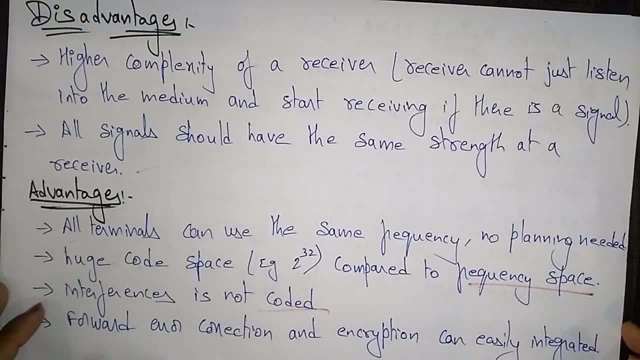 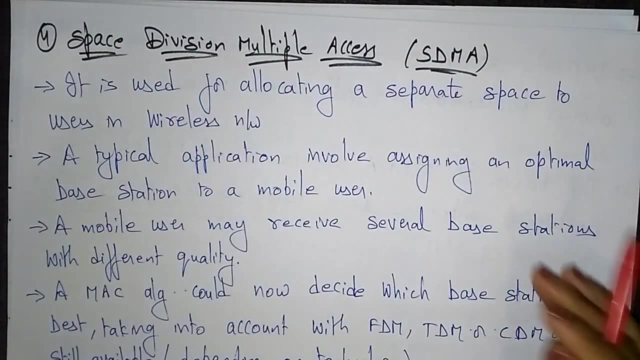 compared to the frequency space and interference is not coded here and forward error correction encryption can easily integrate it. so this is about the cdma. let me explain you. the sdma also the space division, multiple access, the another multiple access technique. this is the last multiple access technique. 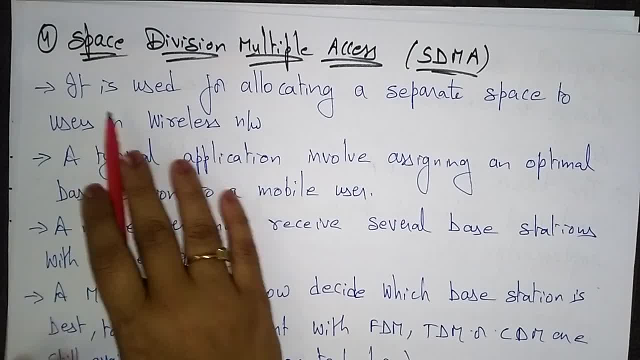 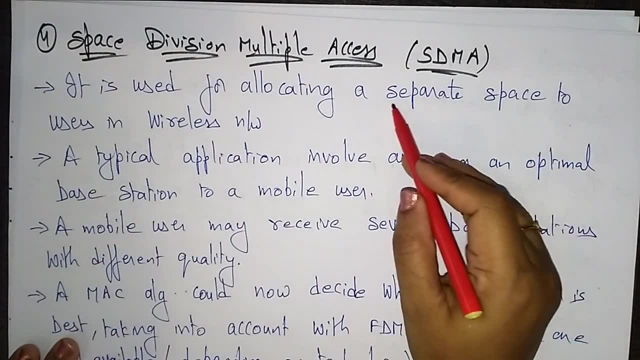 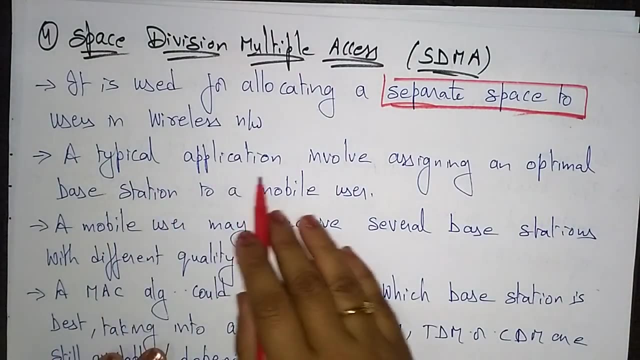 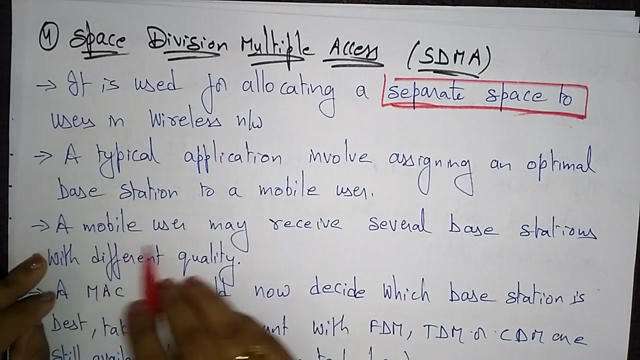 this space division. multiple access is used for allocating a separate spaces to users in wireless network, so it is allocating the separate spaces, a separate spaces, to users in the wireless network. a typical application involve assigning an optimal base station to a mobile user, and here the mobile user. 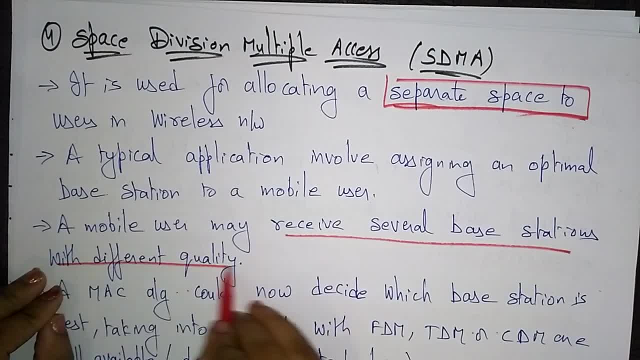 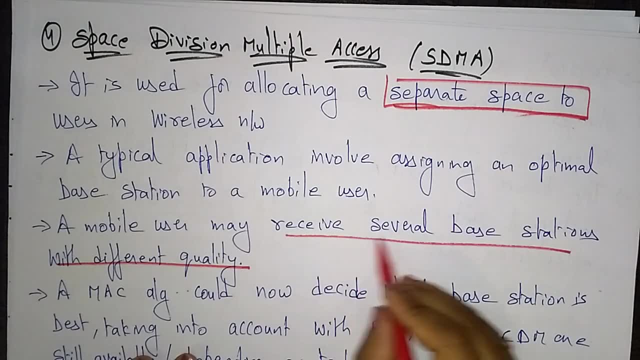 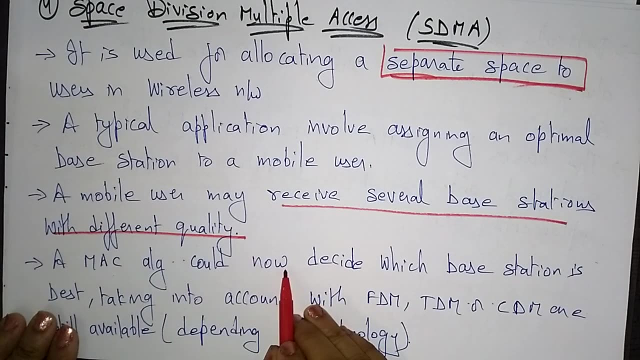 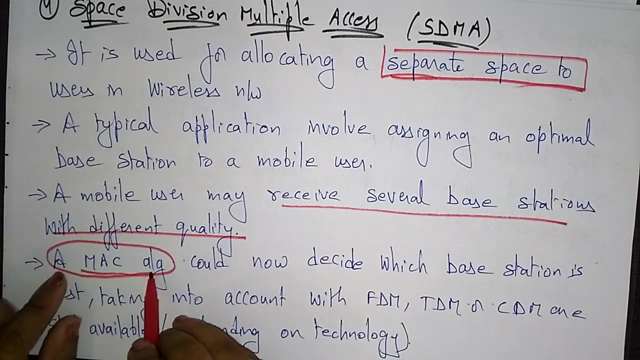 the mobile user may receive the several base stations with the different quality. so, whatever the mobile users here in the that we are using in the space division, multiple access that receives the several base stations with the different quality. a mac algorithm could now decide which base station is the best. so the mac is the main thing- is used to come used for the communication. 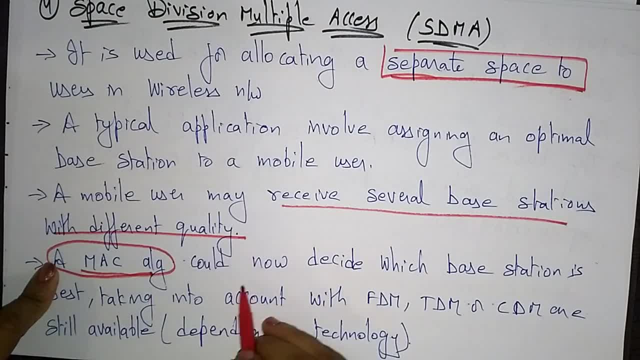 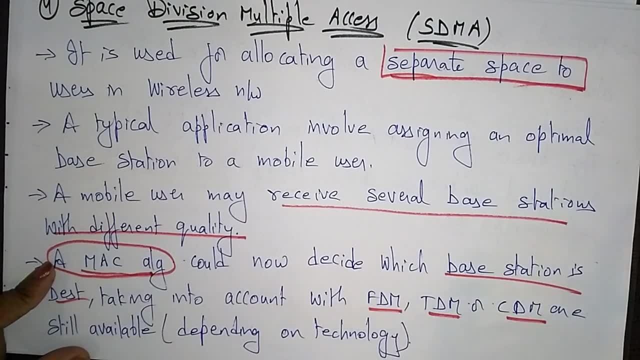 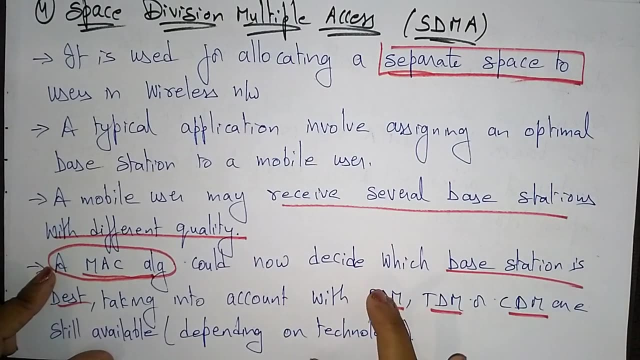 that the medium access control algorithm has to decide which base station is best taking into account with fdm, tdm and cdm. so far you have seen the frequency division, multiplex and tdm and the cdm. so by knowing all these things, the mac algorithm has to be decided which base station is best taking into account of these. 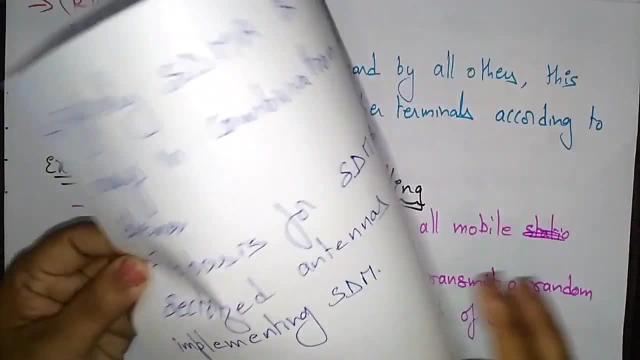 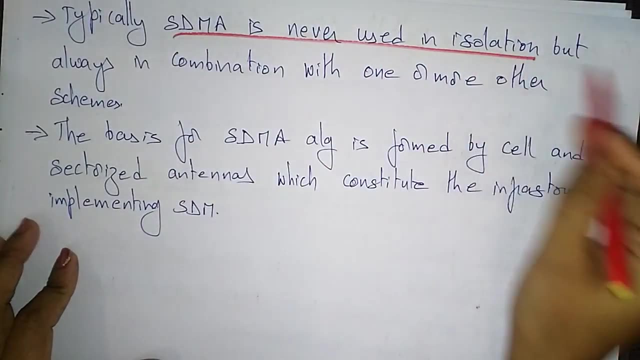 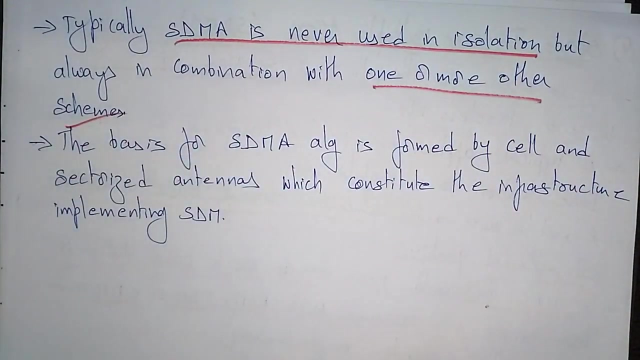 are still available, depending on the technology. so typically sdma is never used in high isolations. there sdma is never used in isolation, but always in combination with one or more schemes. so sdma will not be work on isolation. it has to be combined with some or one or more techniques.